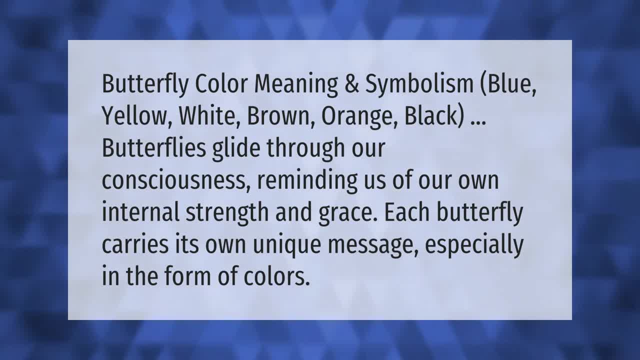 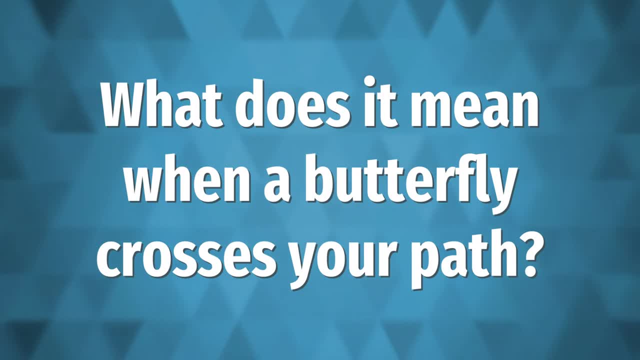 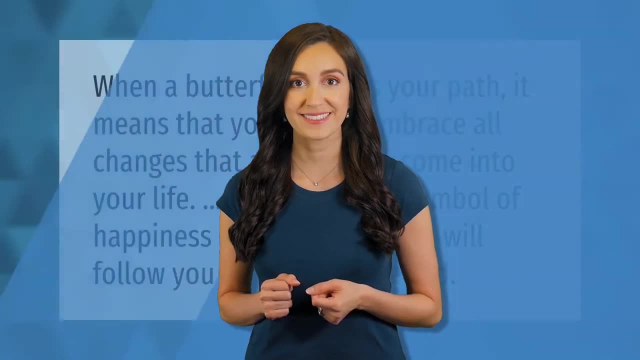 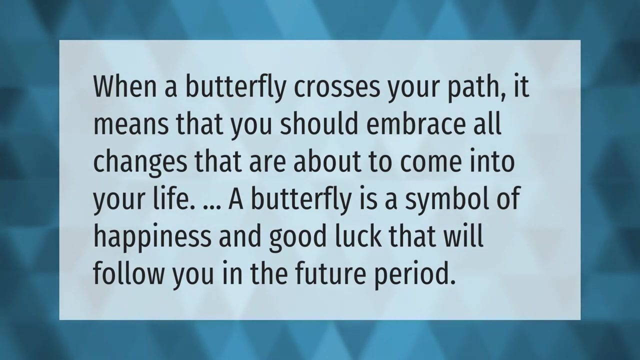 Each butterfly carries its own unique message, especially in the form of colors. Take our lead. Let's help you make your mark. When a butterfly crosses your path, it means that you should embrace all changes that are about to come into your life. A butterfly is a symbol of happiness and good luck that will 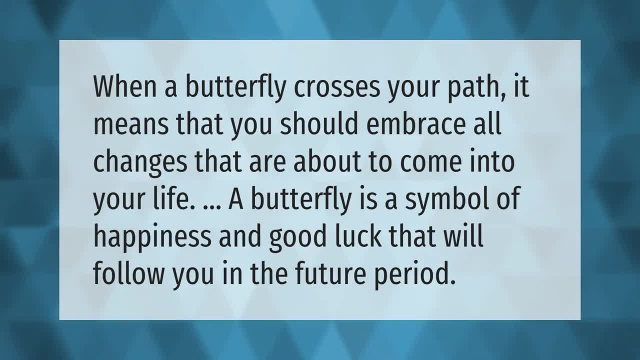 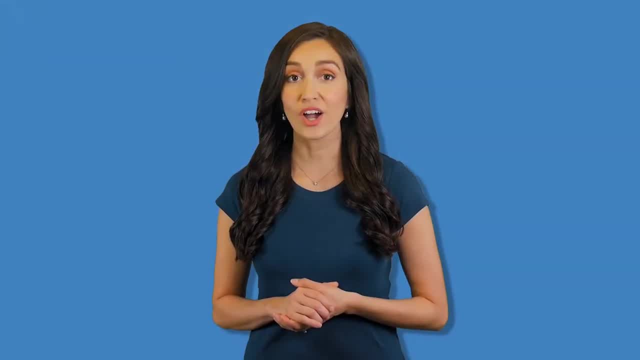 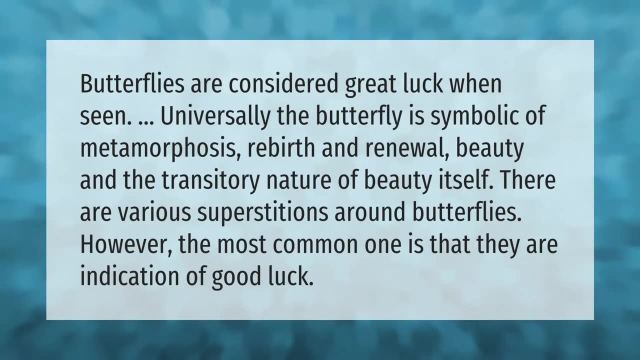 follow you in your life. Take our lead. Butterflies are considered great luck. when seen Universally, the butterfly is symbolic of metamorphosis, rebirth and renewal, beauty and the transitory nature of beauty itself. There are various superstitions around butterflies. However, the most common 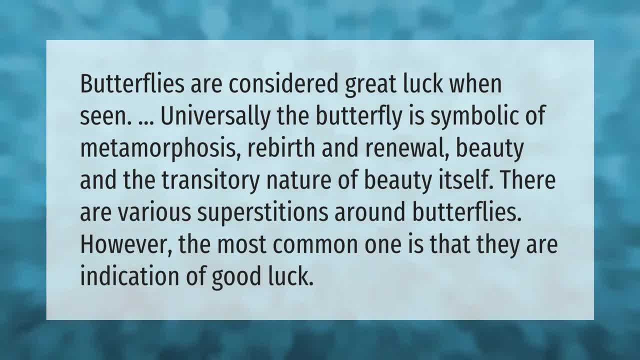 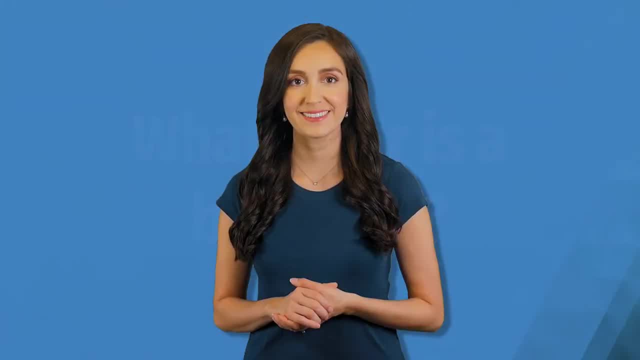 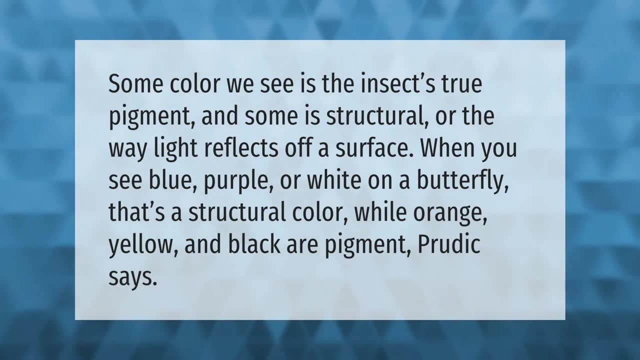 one is that they are indication of good luck. Take our lead. Some color we see is the insect's true pigment and some is structural or the way light reflects off a surface. When you see blue, purple or white on a butterfly, that's a structural color. 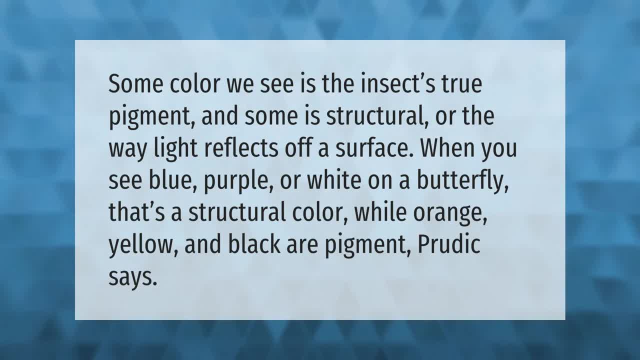 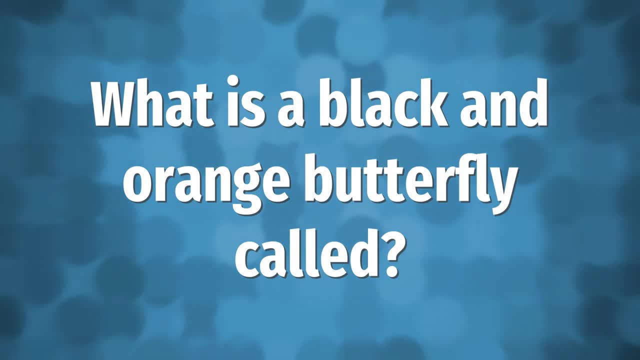 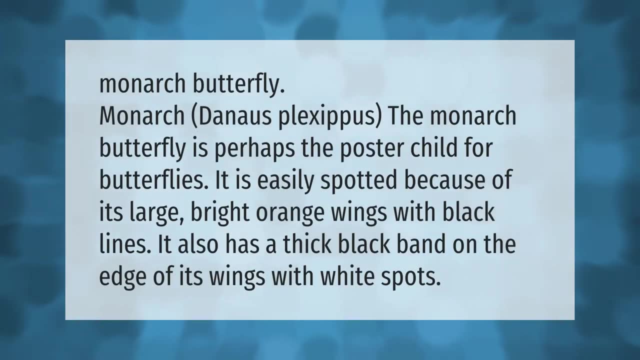 while orange, yellow and black are pigment. Prudik says: Make your mark, Take our lead. Monarch Butterfly. Monarch Dyn bulderpaus. The monarch butterfly is perhaps the poster child for butterflies. It is easily spotted because of its large bright orange wings with black lines. It also has a thick black band on the end of its wings, which means it is easy to recognize mixing colors off projektors. 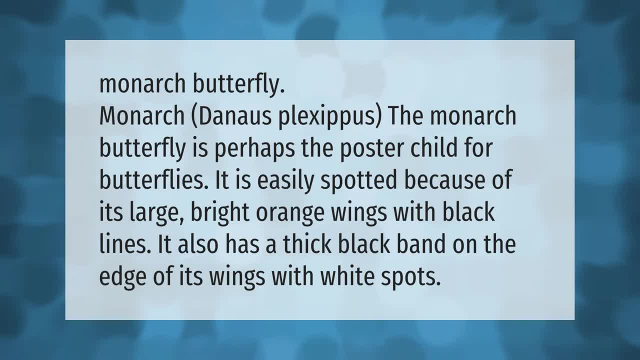 It is Lucera Budapest and would be very useful to succeed with防火. Look at Prudik here. Your eyes will acontece, as it will be separated into 2 in 3 areas around your face band on the edge of its wings with white spots. 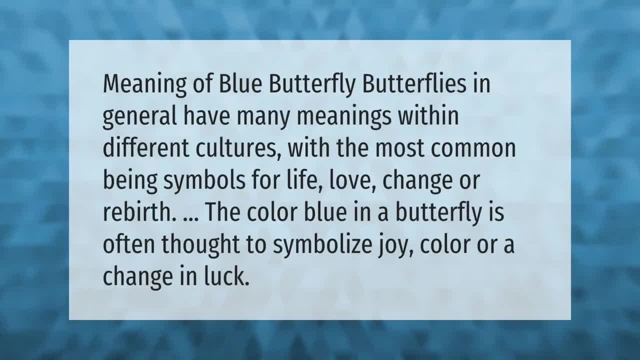 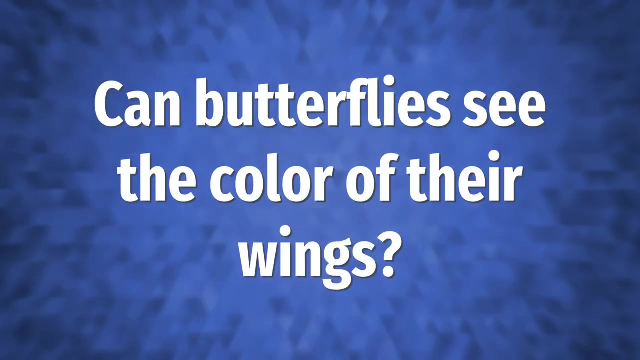 Make your mark, take our lead. Meaning of blue butterfly. Butterflies in general have many meanings within different cultures, with the most common being symbols for life, love, change or rebirth. The color blue in a butterfly is often thought to symbolize joy color or a change in luck.